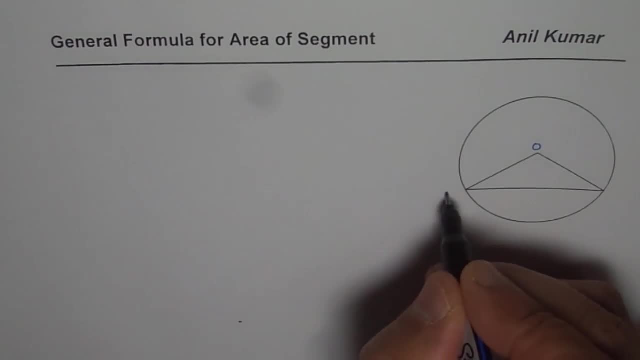 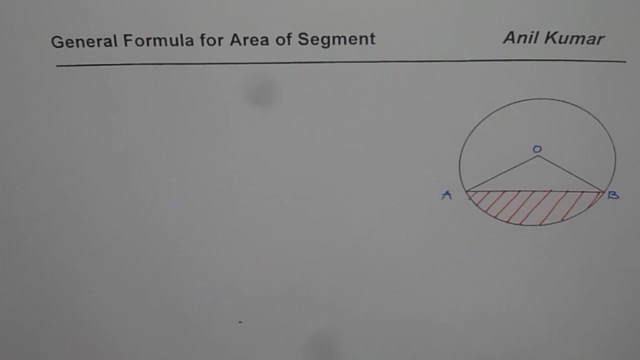 What center? let us say O and we have this chord AB. Then area of the segment is the area enclosed between the chord and the circle, So that area we are interested in finding. So let us see how to develop a relation for this. So basically, the area of this segment. this is called the segment. Let me write down segment here. 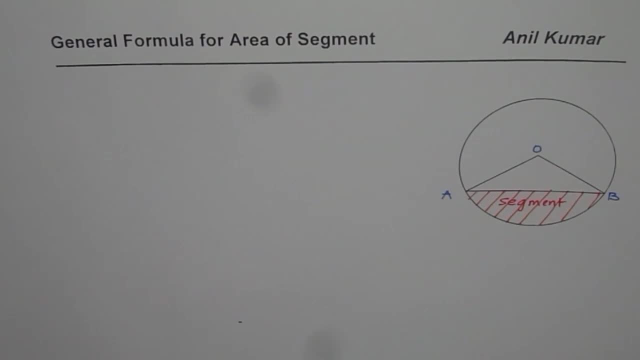 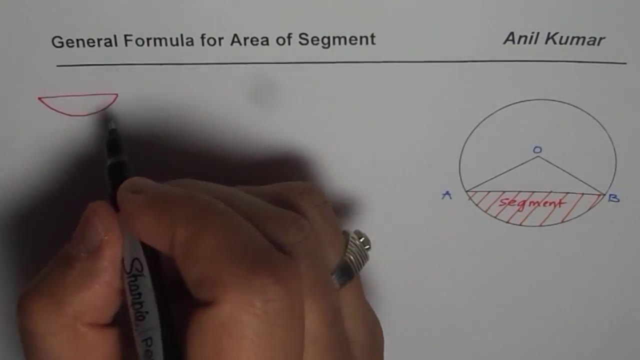 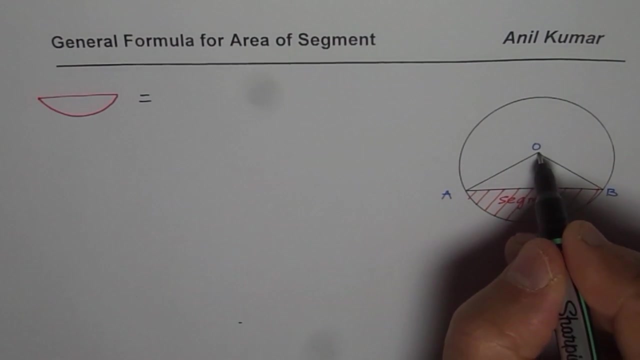 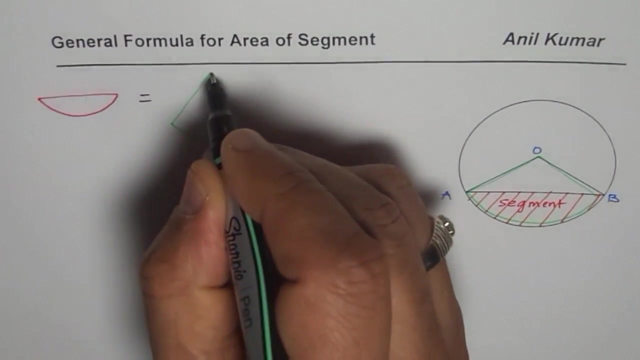 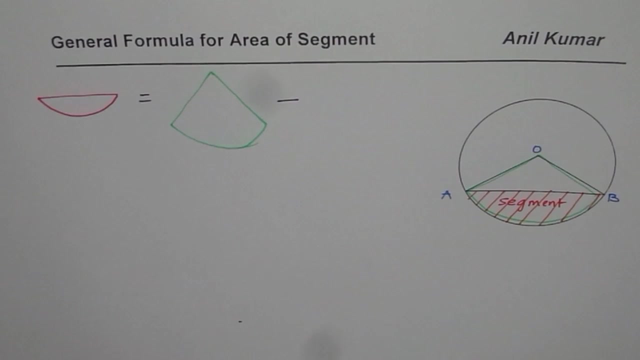 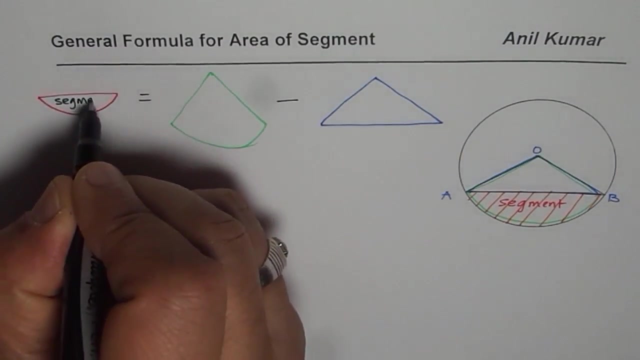 So area of the segment which is, let us say, like this in this particular case, is equal to, let us say, area of the sector, which is kind of like this: Do you see this whole area? So it is the area of the sector, Area of the triangle. So let me say, that is my triangle, Okay, So area of triangle. So that is the formula which we want to derive. So area of segment is equal to: So this is the segment, This is the sector And that is a triangle. 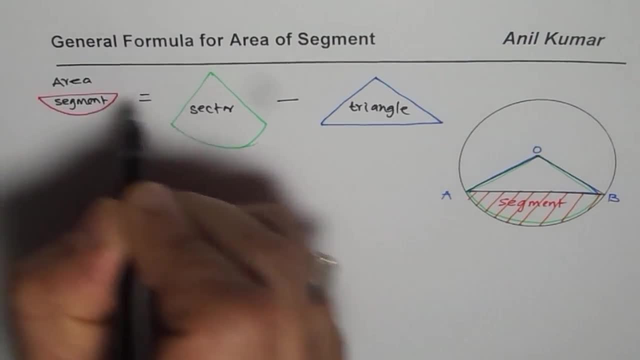 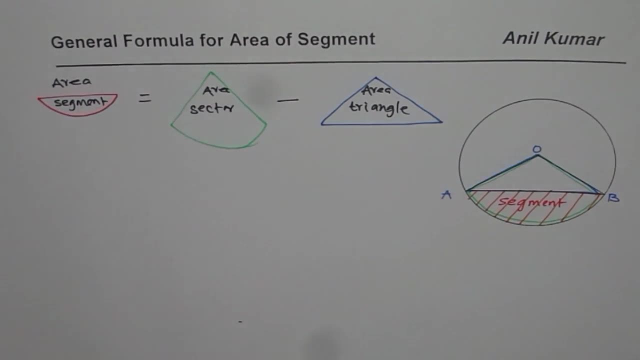 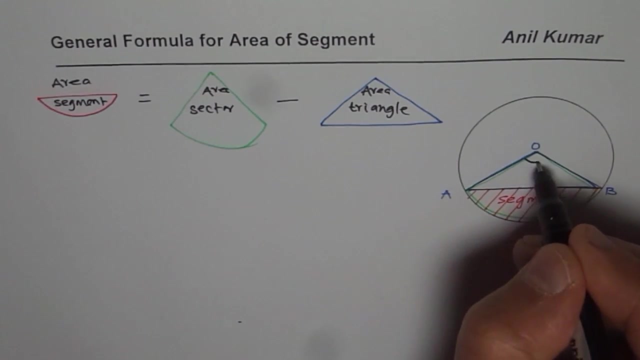 So this is the sector And that is a triangle. So this is how their areas are related, right? So I hope now it's absolutely clear. Now to find the area of the sector, it is the ratio of total area to the angle enclosed. So if 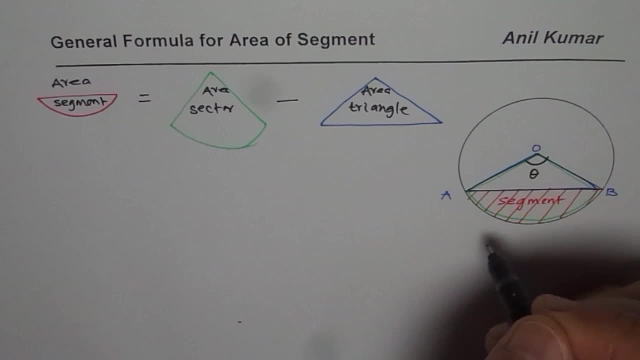 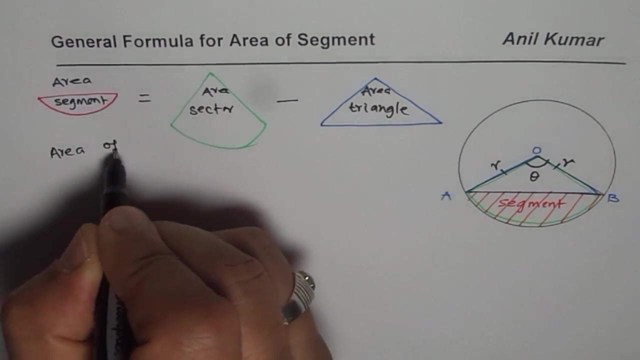 let us say this angle is theta, then it is termed in terms of angle To find the total area. we should know the radius of the circle. So that should be the radius, correct? So that is the radius. So first let's say area of sector. Area of sector is what Is area? 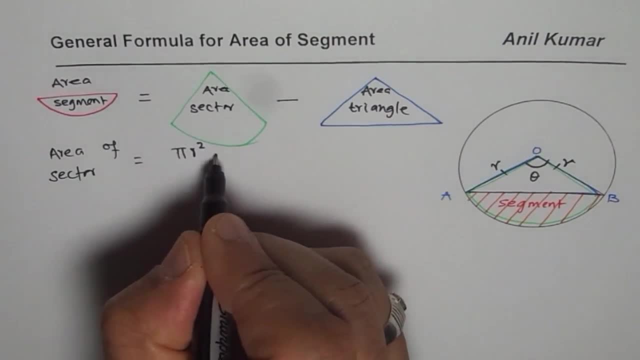 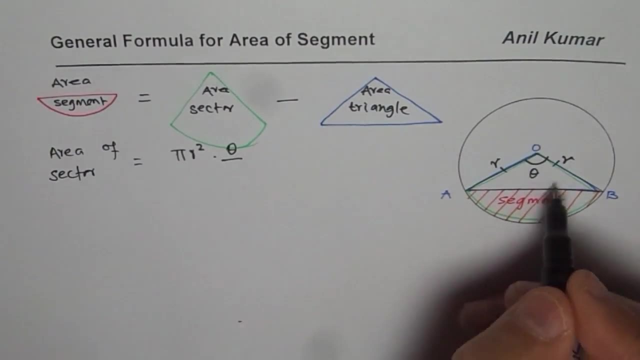 of the whole circle, which is pi r squared times ratio of this angle. If this angle is smaller, the area is going to be smaller right To the total circle area. So if you are doing it in radians, then it should be 2 pi, correct? So? and if you are doing it, 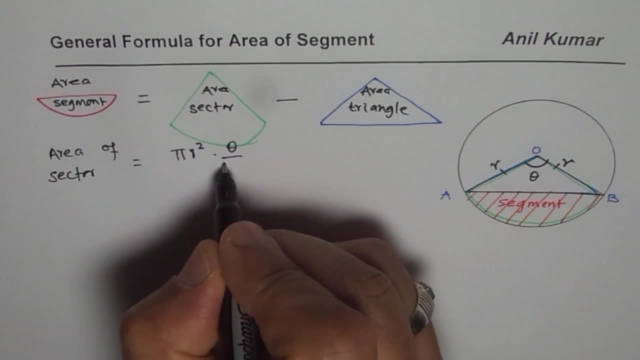 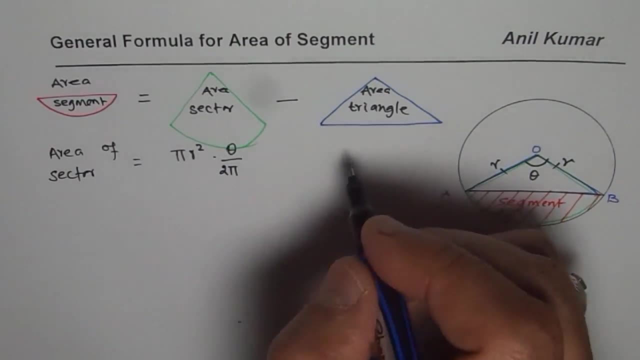 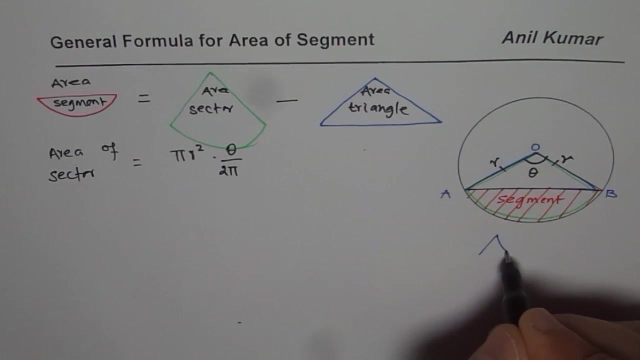 in degrees, it should be 360.. So this time I will take 2 pi in radians, right? So those of you who are doing it in degrees, for them this formula will be equal to. so we will write here, right So the sector. 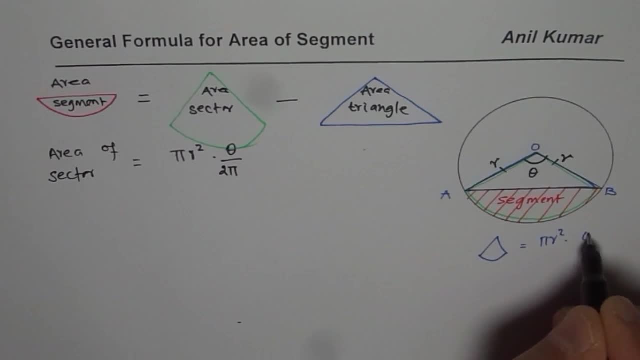 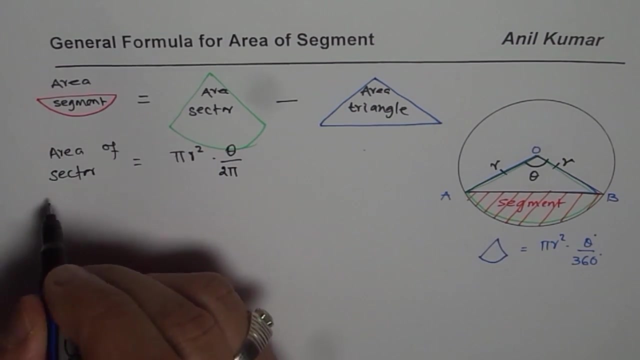 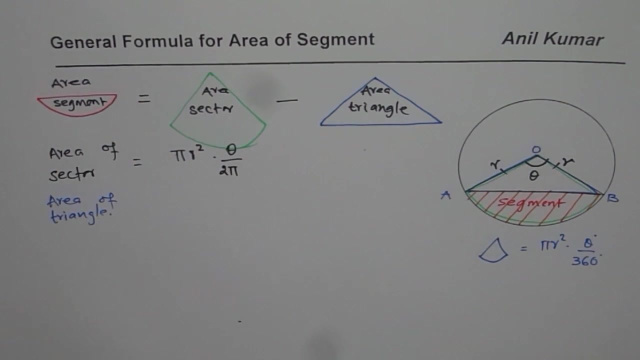 which is kind of like this will be pi r squared times theta over 360 degrees. okay, If you are taking in degrees. okay, Now the other thing is area of triangle. Now, area of triangle is kind of tricky here. How to find area of the triangle? Now to find area of the triangle. 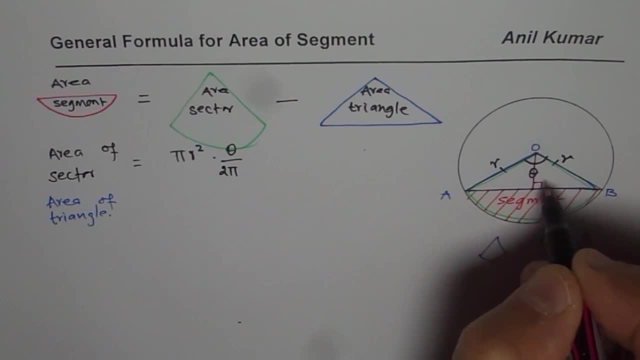 you have to draw a perpendicular from the center. As soon as you draw the perpendicular, these two sides will be divided into two equal parts and the angle will be divided into half. So we have theta by 2.. Do you see that, Once you know this theta by 2 angle, in that case, 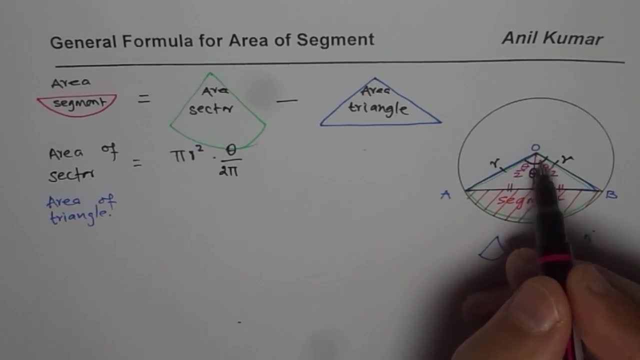 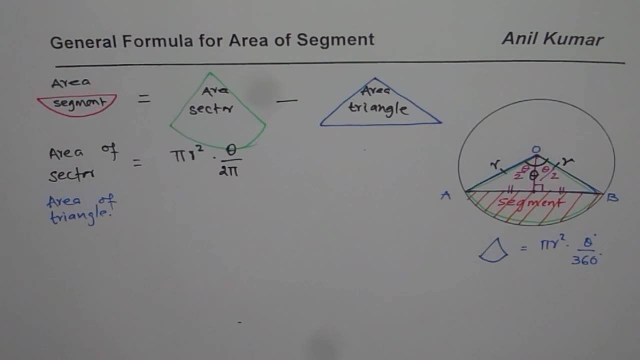 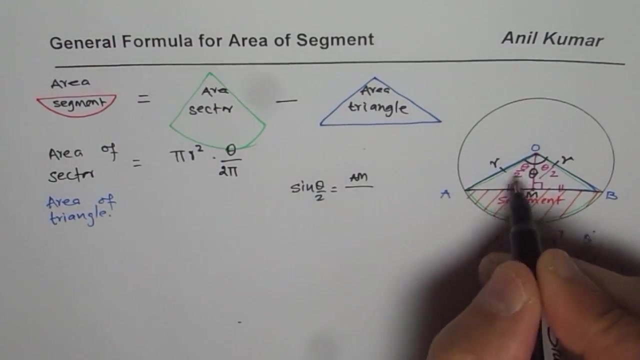 you can write opposite side and adjacent sides. Adjacent side is your height in terms of theta and the angle, and you can find all other points. So let's call this point as the midpoint m right. So now, from here, what we can say is: sine of theta by 2 will be equal to a m over. 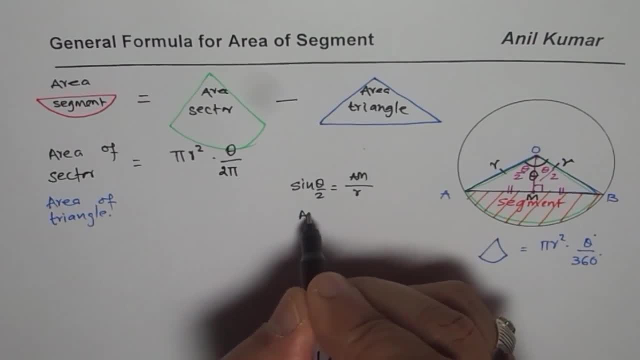 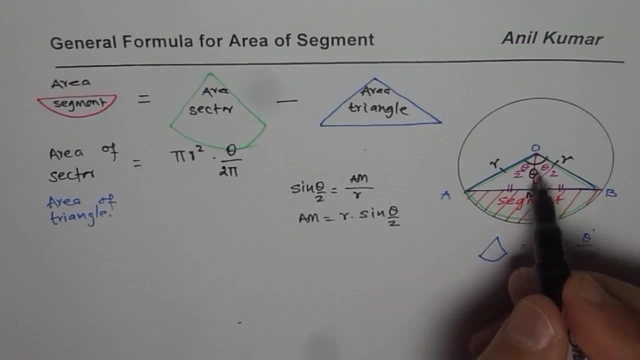 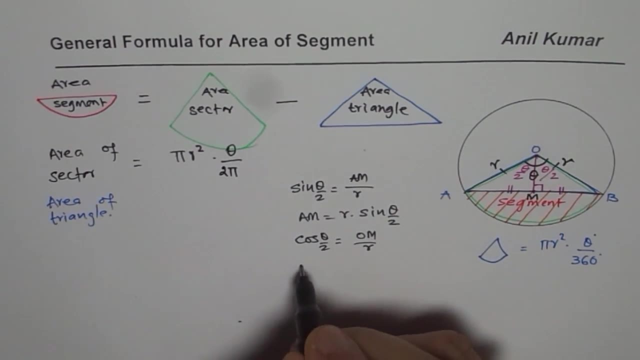 2, right. So we can say a m which is half of theta by 2, right. So we can say a m which, and we can find what om is from cos theta by 2, right, cos theta by 2 is om by r or om equals to. 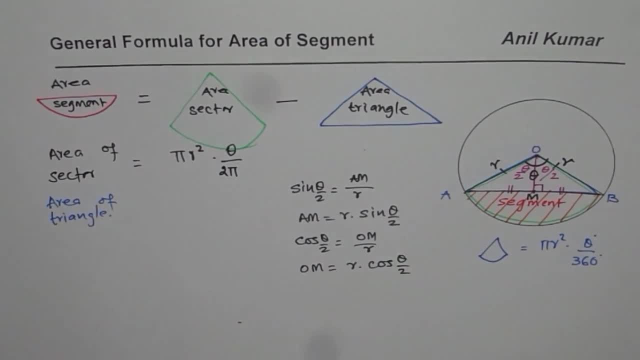 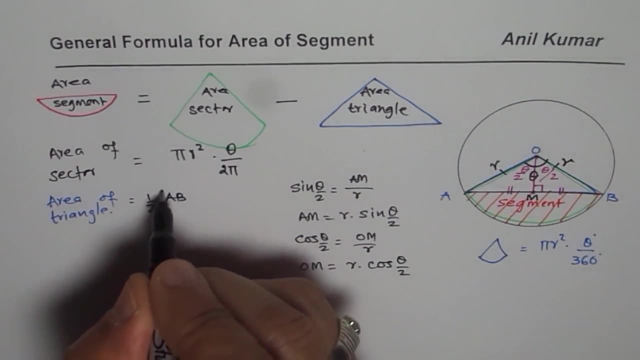 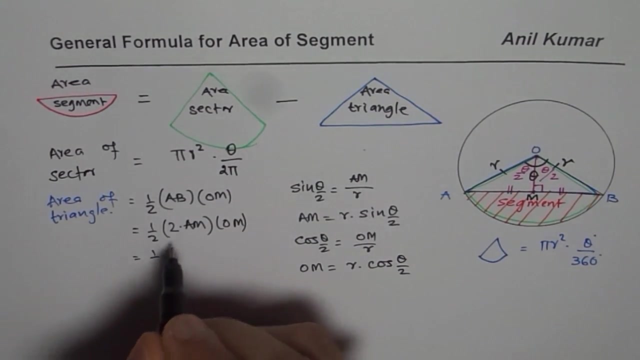 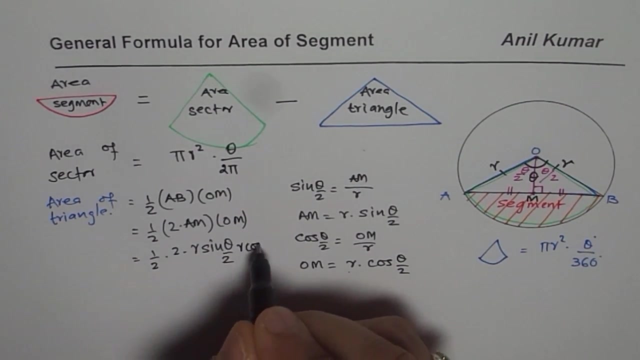 r times cos theta by 2, correct. so area of triangle will be half ab, which is the base times om, which is the height. now ab is 2 times am, right, 2 times am times om, correct. now we have half 2 times am. am is r sine theta by 2, r sine theta by 2 and om is r cos theta by 2, r cos theta. 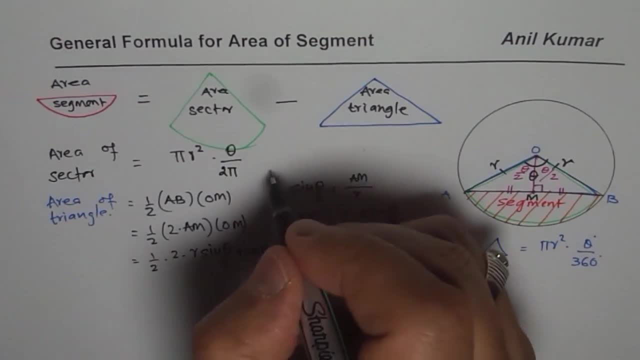 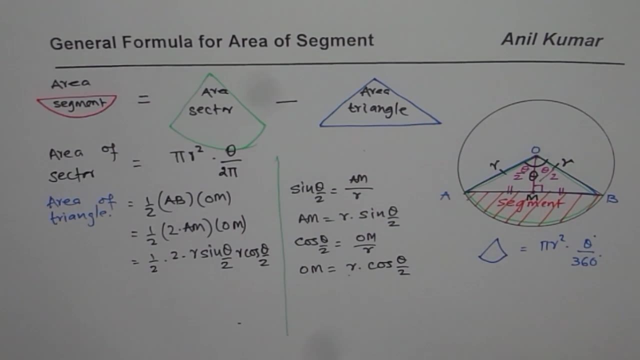 by 2, right so? so that is how you get area of the triangle. you get the point. so this is, this is the formula. so now we can kind of simplify this and then write down the formula itself, which is: equals to r square sine theta by 2 times cos theta by 2. at times you know the formula. let me use one more. 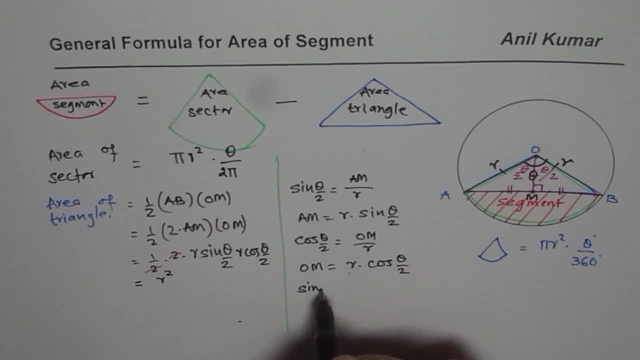 relation here. we know sine sine 2a equals to 2 times sine a cos a right. some of you know this formula, so so theta by 2 will give us theta provided we have two times. so we say we could simply r times r is r squared divided by. 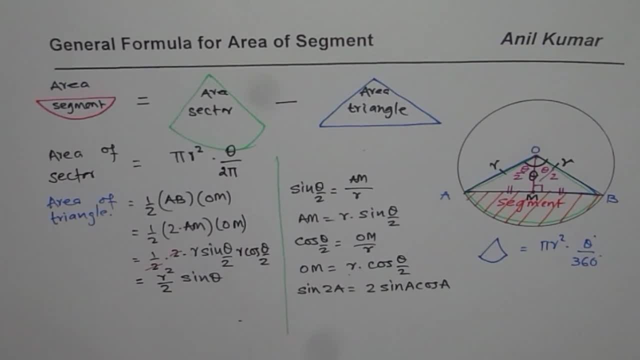 2. we could write this as sine theta also, so so that is how you can get area of triangle from here, correct. or you could write in theta by 2. it's one and the same thing, but you can write the formula. ok, now we know area of triangle also, which is r Squared by 2, sine theta, in this particular case, area. 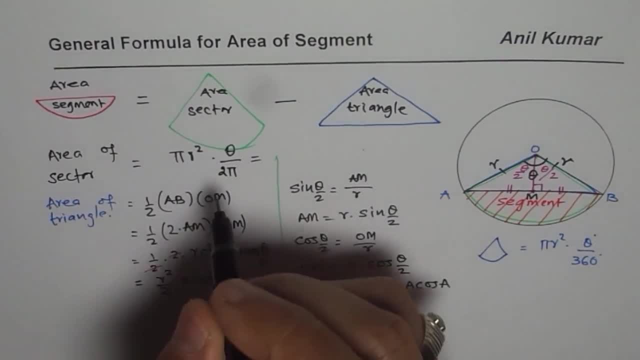 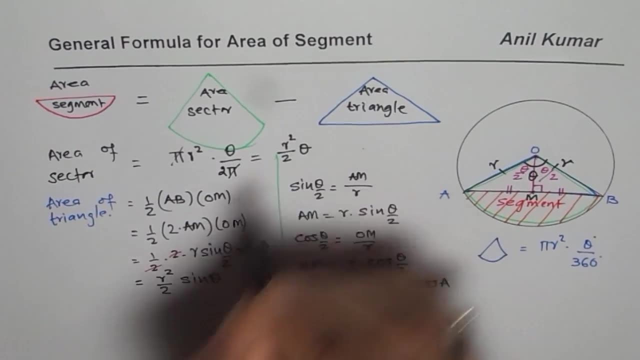 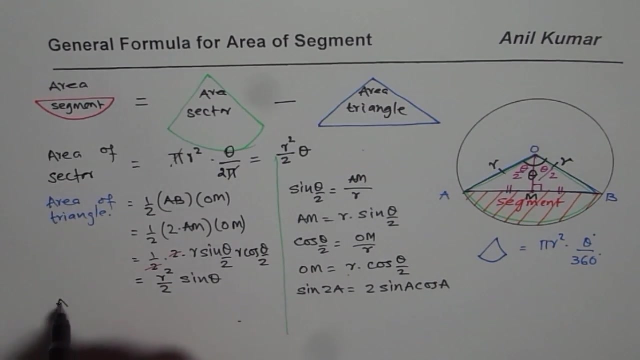 of the sector. let me simplify this part also: store pi, pi and pi cancels out, so we get r Square by 2 theta. do you see that? so that is what we get now. we will write area of segment, so we have area of segment, and cancels out. that is understand. so we have area of segment. so triangle star is equal to the area of.